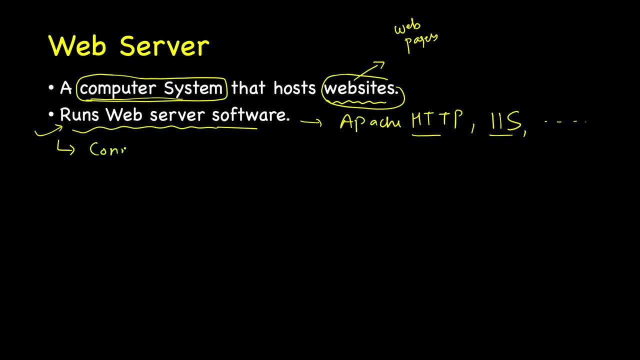 this computer system should be connected to internet in order to act as a web server. Otherwise, clients- web clients- cannot contact it through HTTP, So it may not be able to. it will not be able to serve those, So it will not be acting as a web server. So it should be connected to internet And it should be running a web server software. So typically web servers host multiple websites. Some only host a few, while others may host some. 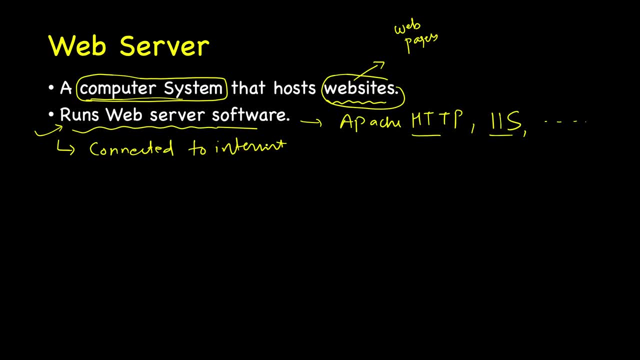 Several hundreds, But there are some dedicated servers also. So, based on that, we will categorize a web server into two parts. One is that web servers that host websites for multiple users- These are called shared hosts- And there are some dedicated web servers that will be hosting websites for single person or company, And these will be called 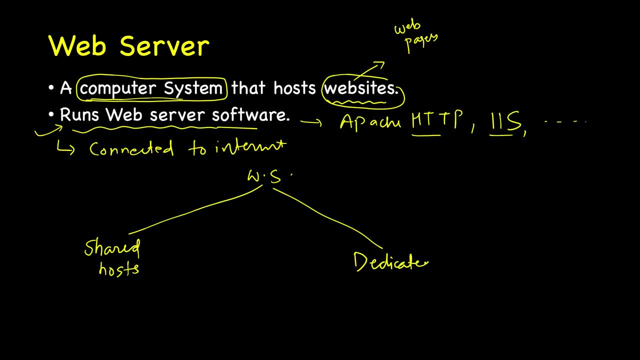 dedicated hosts, So which servers are shared and which are dedicated. So when, let's say, there is some personal website or some small websites which does not have huge amount of traffic, then those will would be generally hosted on shared hosts. But if there is a huge website and it has high traffic, then that requires 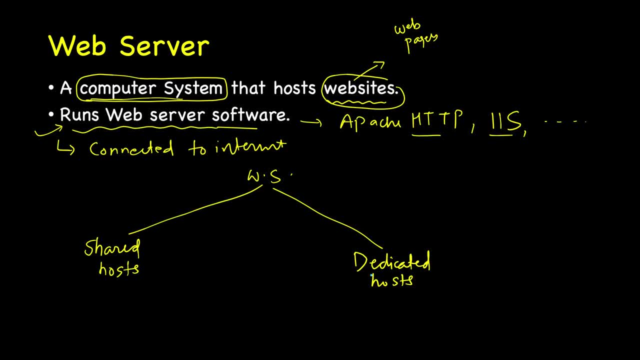 a dedicated server for that, and also if a website is running technically on a shared host site, if the site requires custom servers modification, then it will go for dedicated hosts. Then it will go for dedicated hosts. Apply the command meetings of a project. Now let's understand how this web server works. 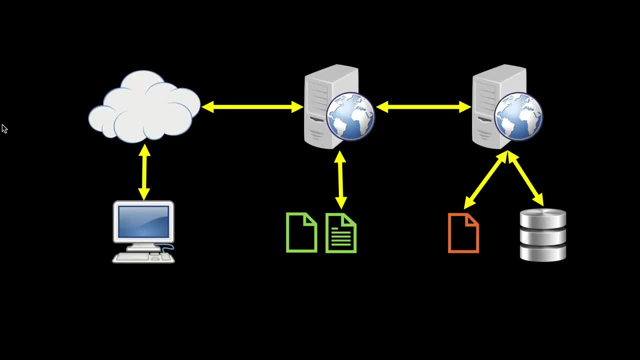 Зайти и защищぐ. So if we have the web server, then there must be a client. So if we have the web server, let's say: this is the web server. So if we have the web server, then there must be a client. 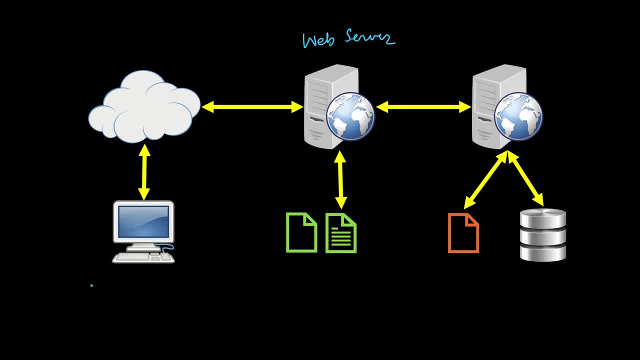 client whom the server is serving, then this client sends an HTTP response from a server, duplicated a client, So we will call it Lyric. So this client sends an HTTP response, Generate a service request to the web server and it will request for some page or it will require. 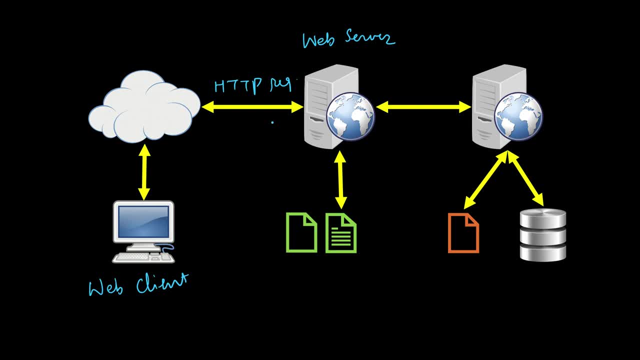 for some other resources. so there are two possibilities. one possibility is that the requested URL, the page that is requested or the file that is requested- is present with the web server. then it will immediately send HTTP response with the file. but it may be possible that that is not present on the web server. so 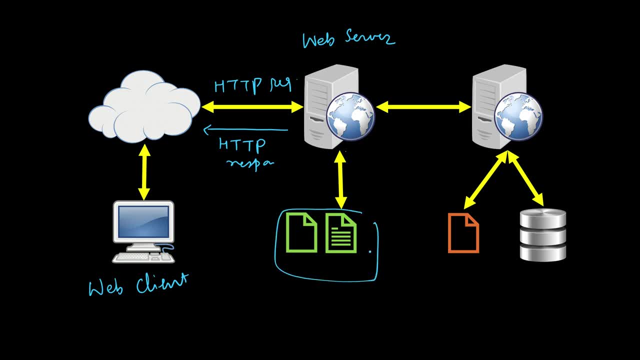 it can look into a static database, so these are files. that is present to this. then there may be also static database which the web server can contact and fetch the file and return to the send HTTP response. but there may be scenario that this is not present in the static DB but it needs some processing. then what this web server 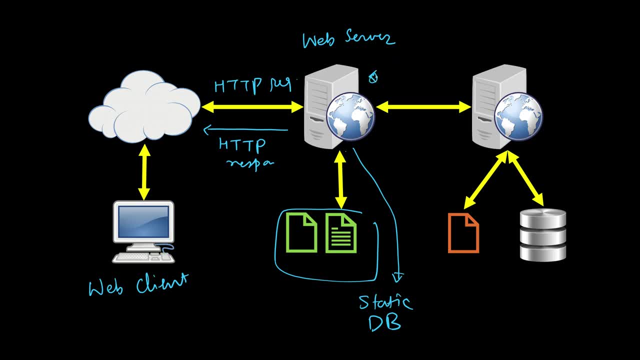 will do is that it will send a servlet request to the application server. so you can now see application server coming into picture. so it will send a servlet request to application server. so just a quick info. what is a servlet? if you may be wondering, a servlet is a small Java program that 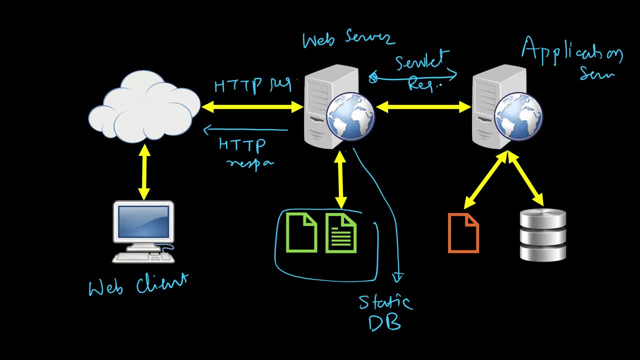 runs with a server that runs with a server that runs with a server that runs with a web server. servlets receive and respond to requests from web clients, usually across HTTP, so these will be some Java programs so it will require some processing, so it will send this servlet request to this application. 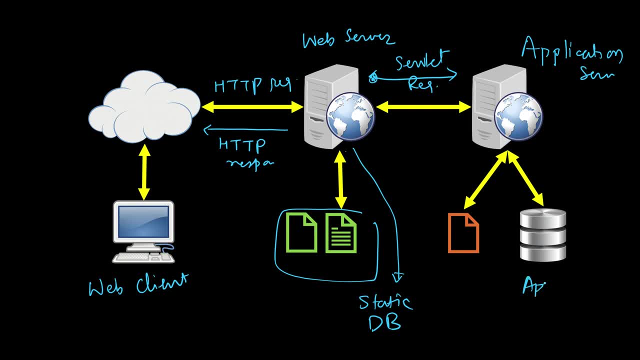 server. it will contact the application data store in order to process, run this servlet and fetch some details from here and do further processing and then it will send it serverlet response to the web server. and now this web server has the response built-in, so response ready so it can send a http response back to the web client. so this is how web server works. 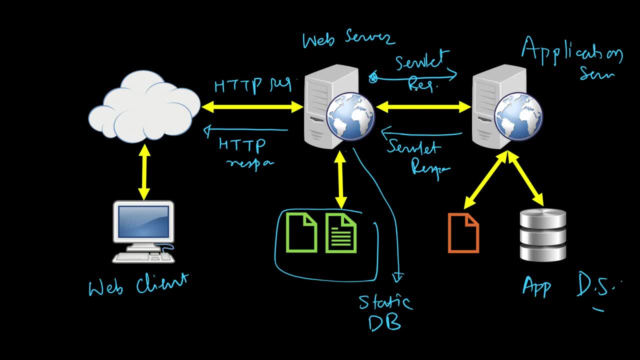 and this application server may not be always required, but it may be required when some intense processing is required which web server cannot handle. so this is a rough idea and you should understand this flow. now let's see some of the examples of web servers. so one most popular. 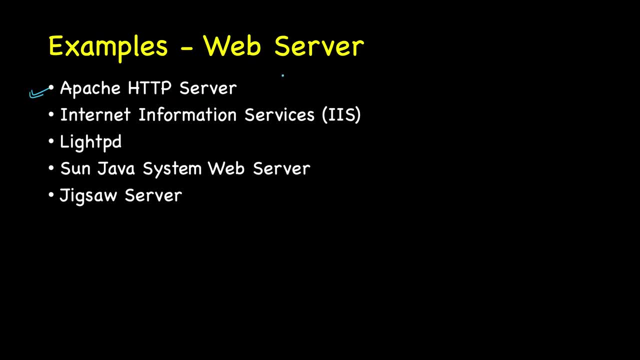 web server is Apache HTTP server and it's the most popular as of now. it's developed by Apache Software Foundation and, just a rough estimate, roughly 60 percent of the web servers run Apache web server and it can be used to run web services which we will be discussing in the next video. so 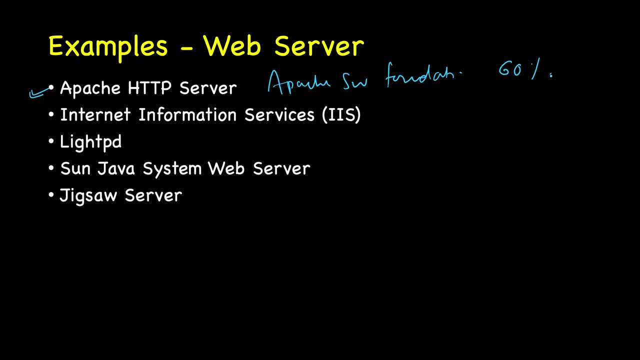 be installed on all operating systems, including linux, unix, windows, freebsd, mac os x and more, and it's a open source software, so all of these are related to its popularity. that's why it's so popular. then we have internet information services, or in short, iis. it's developed by 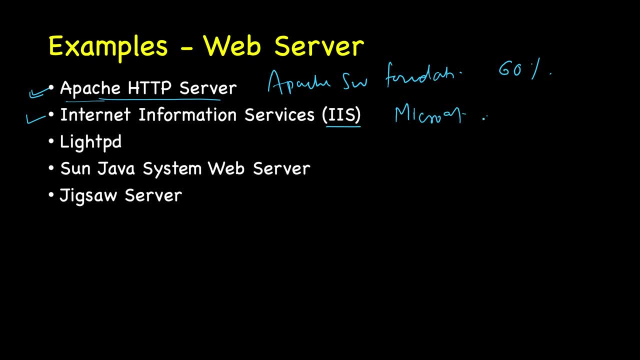 microsoft and it runs on windowsnt 2000 and 2003 platforms and, uh, it is tightly integrated with the operating system so it is easy to administer it. then we have some other web servers, like light, pd, sun, java system web server and jigsaw server. there are a few more, but those are not that much. 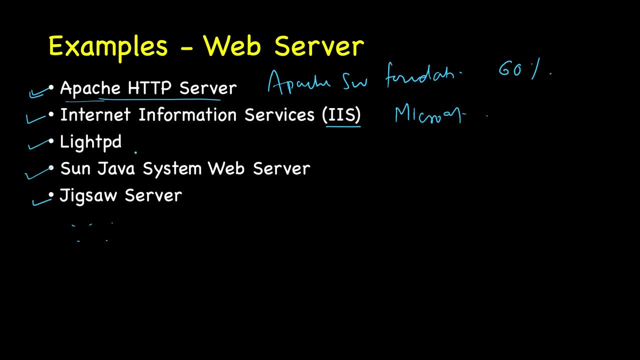 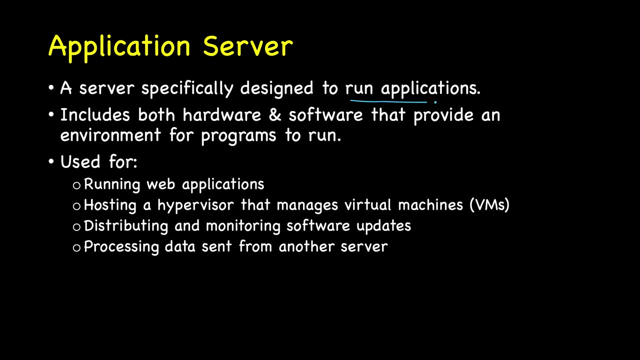 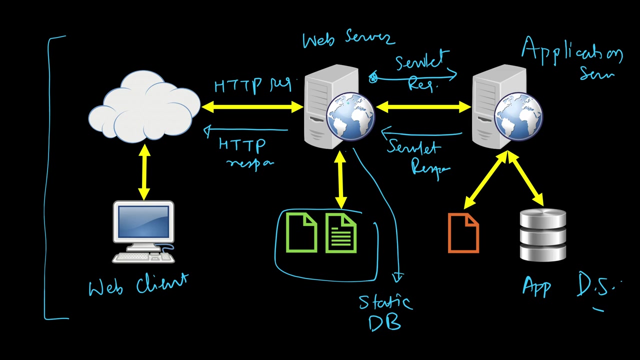 popular. now we have a good understanding of web server. we also know the most popular web servers, how web server functions. let's quickly look at application server. so application server is a server that is specifically designed to run applications, and here also, we had seen that this was coming into picture when this web server did not had the request. 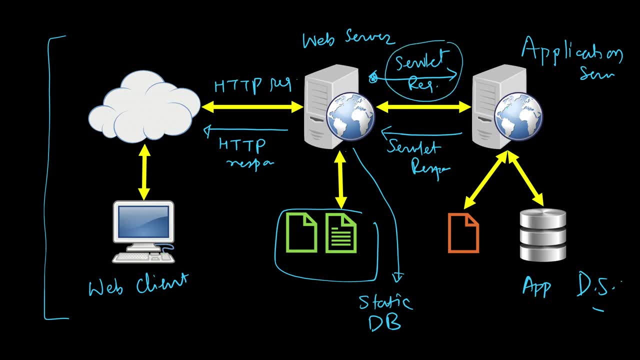 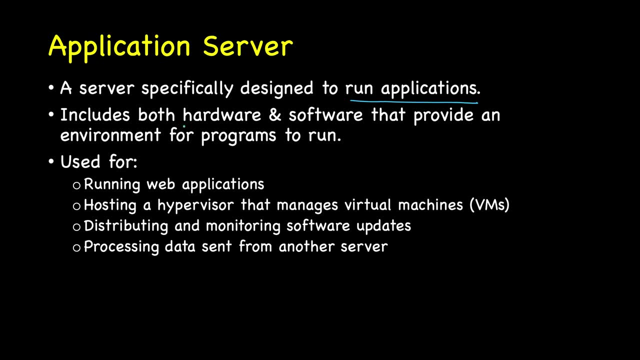 ready and it needed to run some Java program to build the response. so it's a server designed for running applications and it includes both hardware and software that provide an environment for programs to run. so what are some of the uses of application server? it's used for running web applications hosting a. 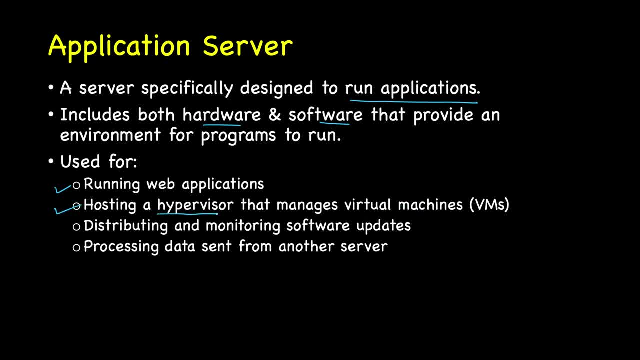 hypervisor that manages virtual machines. so what are hypervisors? these are software programs that manage one or more virtual machines and these can be used to create, start, stop and reset virtual machines. then application server can be used for distributing and monitoring software updates and also processing data sent from another server.